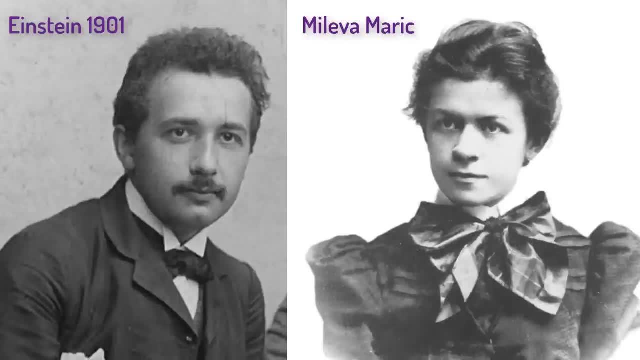 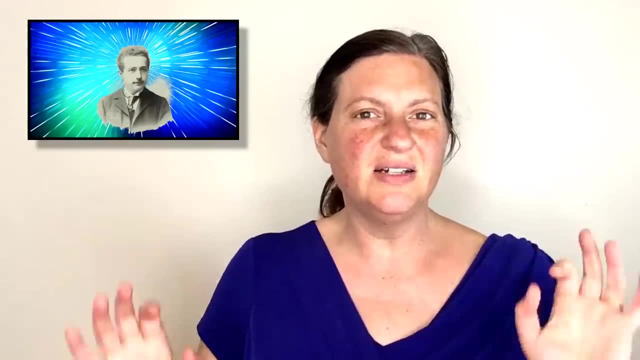 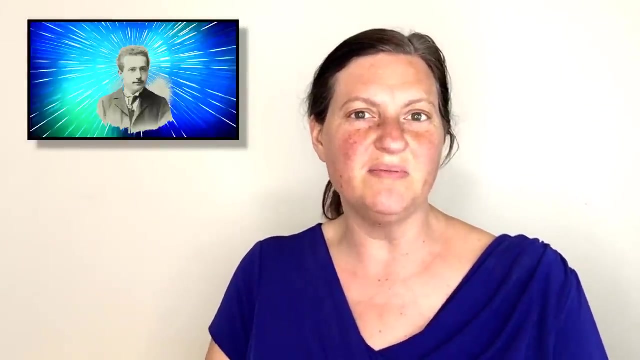 about Max Planck's studies on radiation. misgivings of a fundamental nature have arisen in my mind, so I'm reading his article with mixed feelings. Seven days later, Einstein was still complaining that Planck's idea that the thing that creates light are limited to how they can vibrate was. 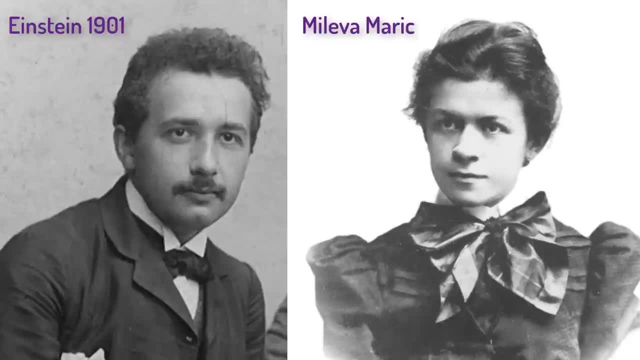 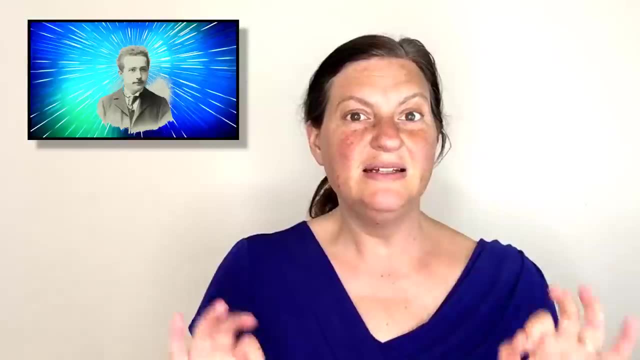 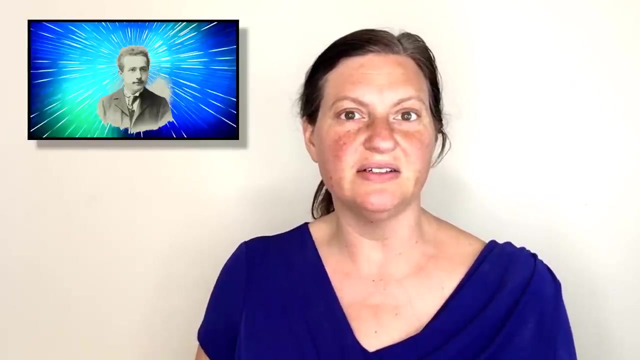 quote an assumption I can't really warm to, and because of Planck quote, my views on the nature of radiation have again sunk back into a sea of haziness. In May I read a paper much more to his liking. A former professor of Mileva's named Philip Leonard had 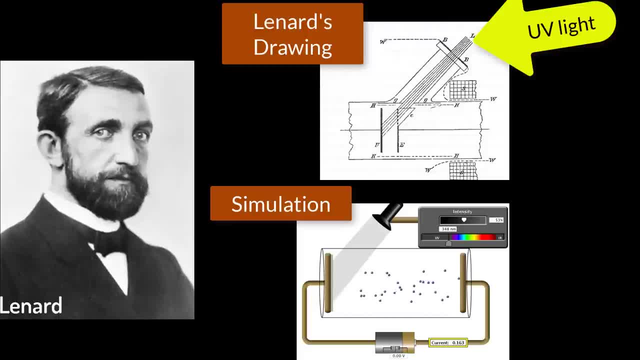 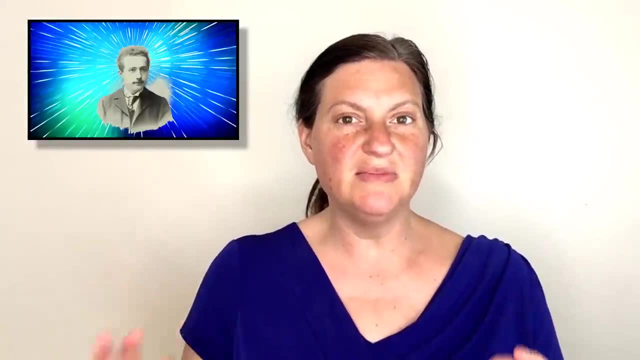 written about an experiment that proved that shining ultraviolet light on a metal plate would cause electrons to fly off the plate. This was only a few years after the discovery that something called cathode rays in vacuum tubes were actually beams of electrons. This phenomenon quickly became known as the photoelectric effect: Photo for light and electric for electric. Einstein. 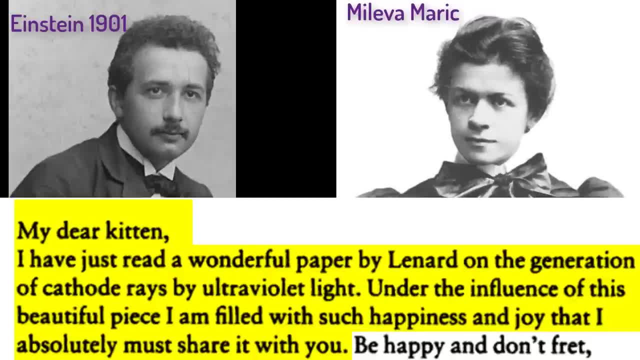 wrote Mileva, my dear kitten, I have just read a wonderful paper by Leonard on the generation of cathode rays by ultraviolet light. Under the influence of this beautiful piece, I'm filled with such happiness and joy that I absolutely must share it with you. There's no hint in this letter. 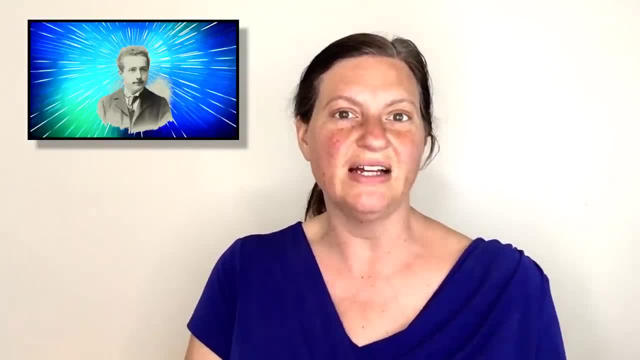 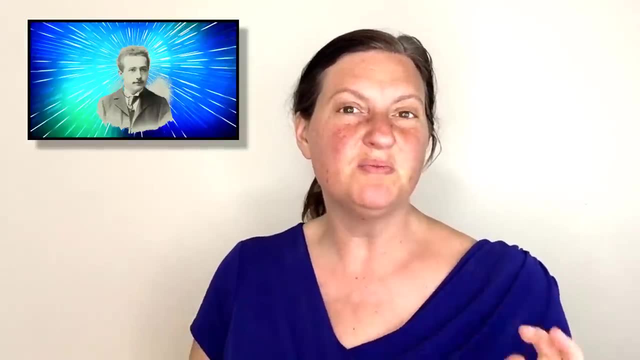 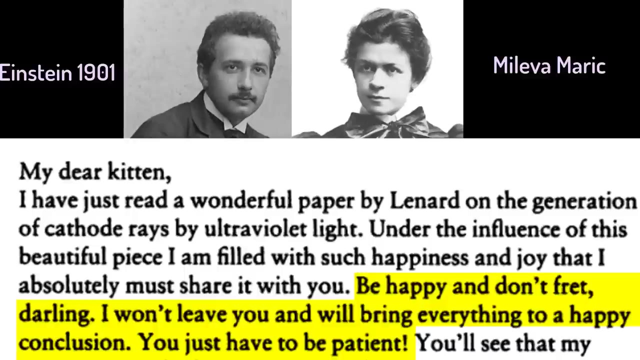 that Einstein saw any connection between the photoelectric effect and Planck's energy bundles. However, Albert and Mileva had bigger problems. Mileva was pregnant with Einstein's illegitimate child. The letter quickly changed from science to comfort: Be happy and don't fret darling. 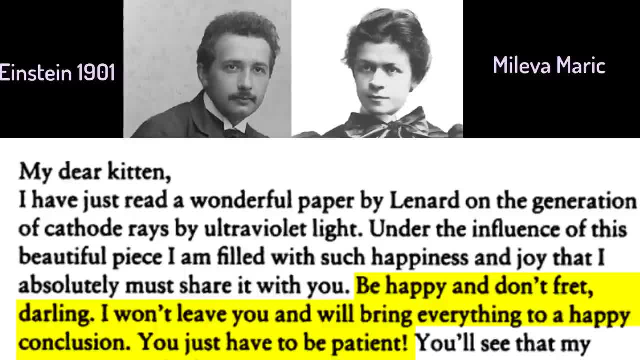 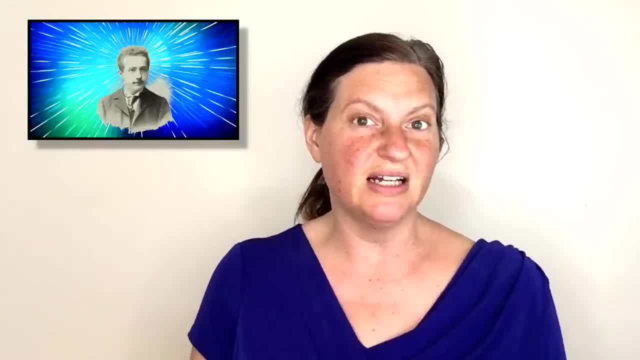 Albert added: I won't leave you and will bring everything to a happy conclusion. You just have to be patient. Mileva had met Albert when she was studying physics at Zurich Polytechnic, and she was one of only 20 women in all of Germany and Switzerland studying science. 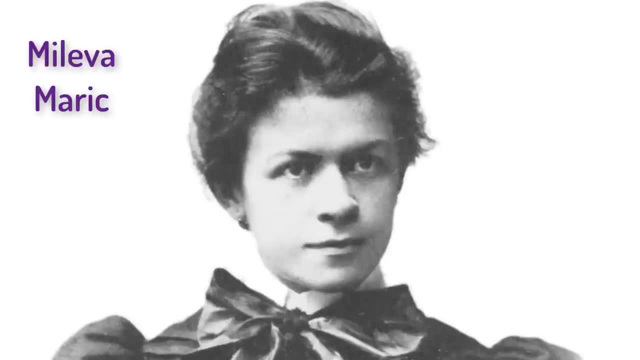 or math. Three years older than Einstein, Mileva had come from Serbia to become a doctor, but had switched to physics. Mileva had been studying physics at Zurich Polytechnic and she was one of 20 women in all of Germany and Switzerland studying science or math. Three years older than Einstein, Mileva had come from Serbia to become a doctor, but had switched to physics. 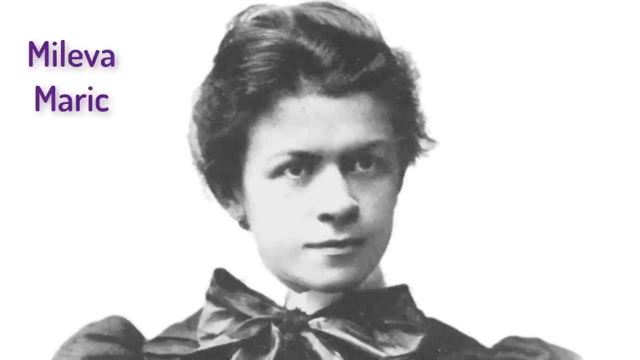 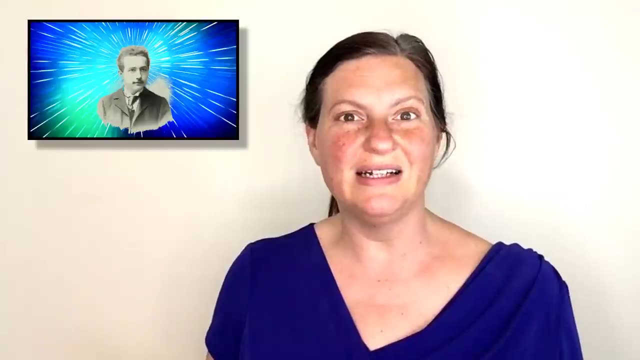 Her grades were fantastic until she fell for Albert then well, not so fantastic. By 1901, Mileva had failed her exams twice, was pregnant and went home to confess her troubles to her parents. Meanwhile, Einstein couldn't find a job, mostly due to his delight in annoying all people in authority. 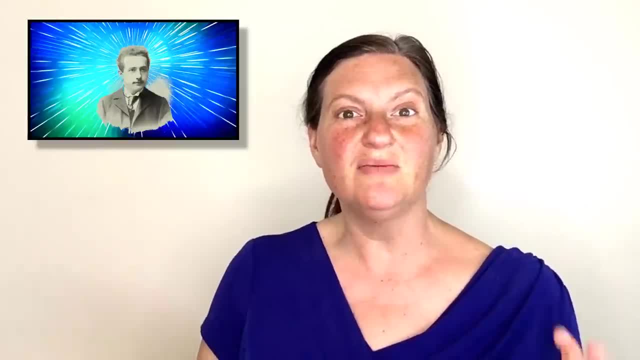 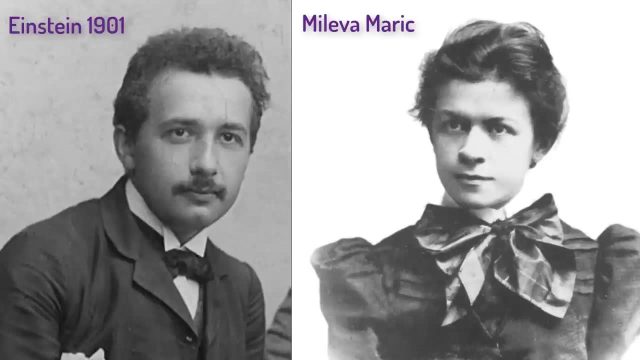 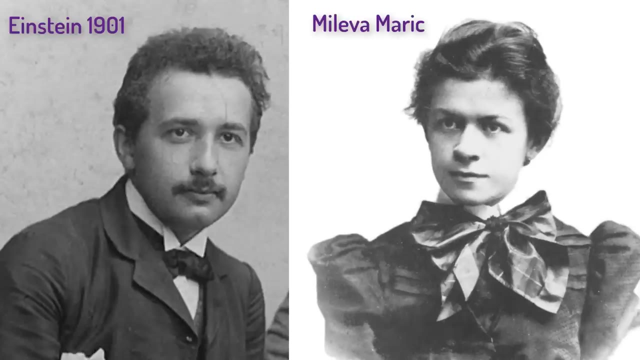 and also due to a small dose of anti-semitism, and refused to marry her without one. Mileva, wrote a friend, Albert has not yet found a job and you know that my darling has a very wicked tongue and on top of it he's a Jew. Don't worry, Albert wrote, I will look immediately for position no. 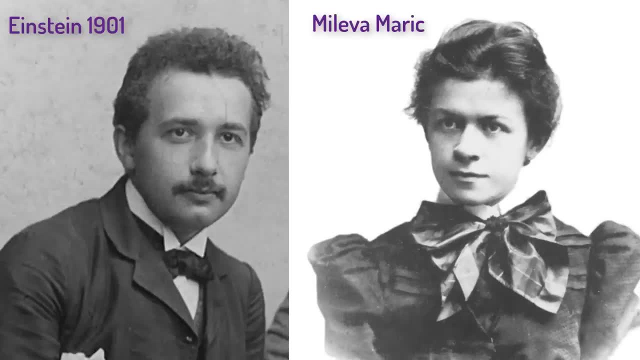 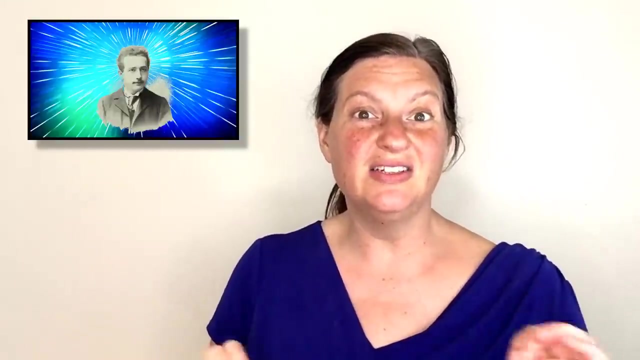 matter how humble my scientific goals and personal vanity will not hinder me from accepting the most subordinate role. the moment I have obtained such a position, I'll marry you. But Albert couldn't find a job or a job he would accept, and Mileva had a daughter, Leserelle, in secret in the beginning of 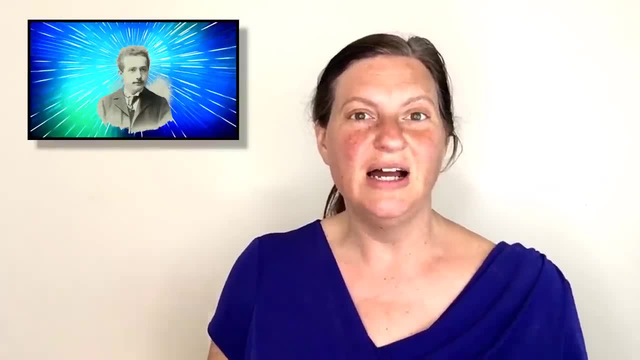 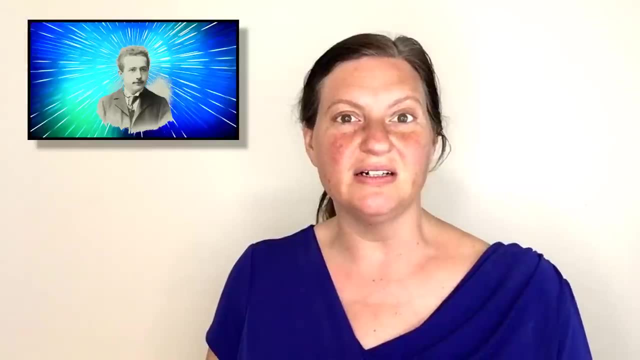 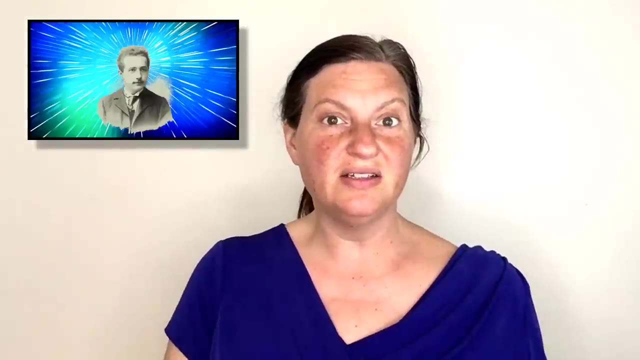 1902.. By June of 1902 he got a job as a patent clerk in Bern, Switzerland, and in January the following year Mileva went to Bern, leaving the baby with her parents, and married Albert. In August, Mileva went back to Serbia and found that she was pregnant again and that their daughter had. 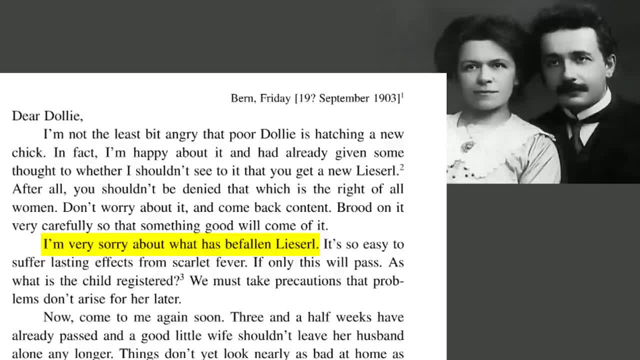 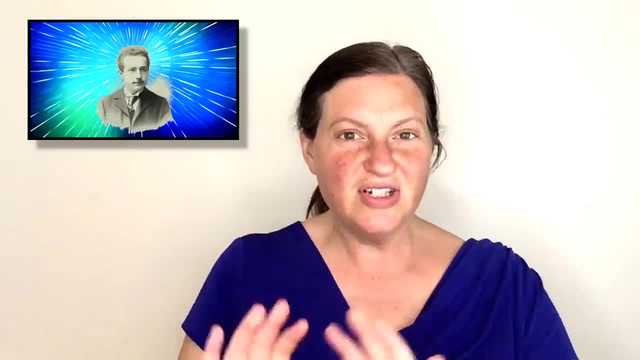 scarlet fever. Albert was mildly concerned about Leserelle, but pleased with the pregnancy, and told Mileva that quote: I'm happy you get a new one. I'm happy you get a new one. I'm happy you get a new one, Leserelle. oi Einstein, darling, you can't just replace babies. He also told her to hurry home. 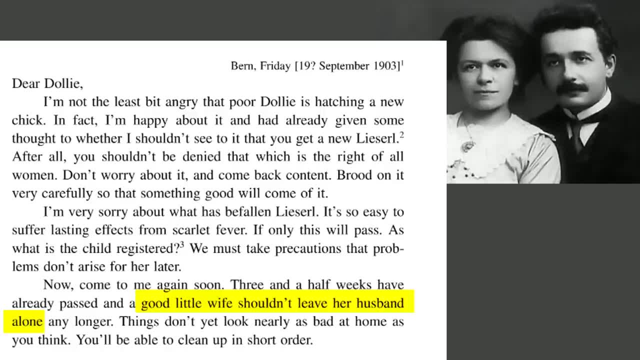 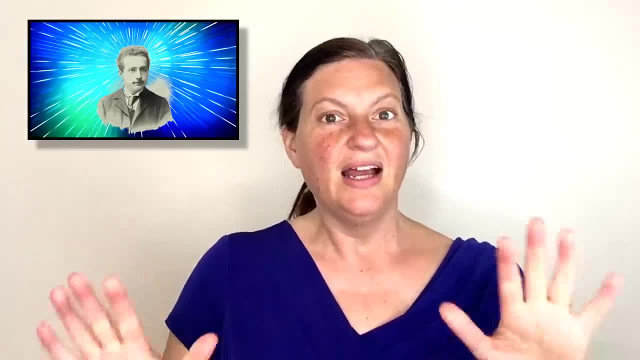 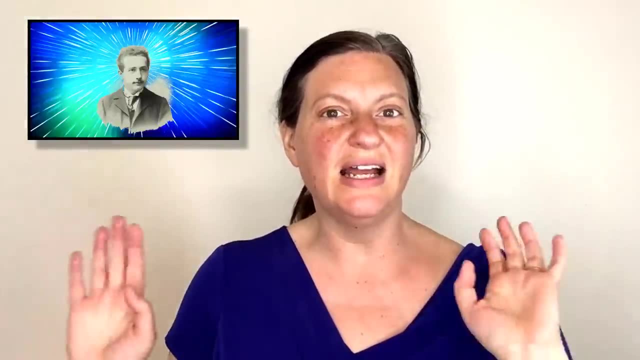 as quote. a good little wife shouldn't leave her husband alone too long. the place was getting messy, but don't worry, quote, you'll be able to clean up in short order. Sigh. Anyway, it seemed like either Leserelle was adopted away or died of scarlet fever, as that's the last that anyone 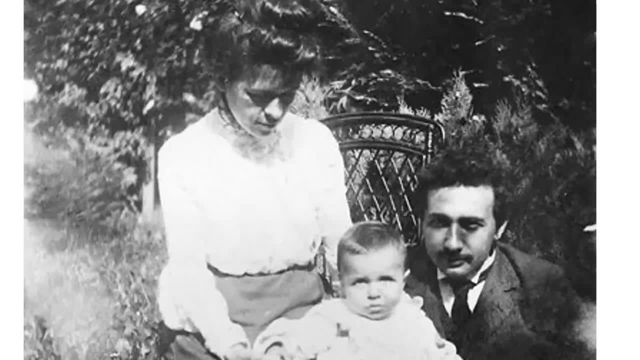 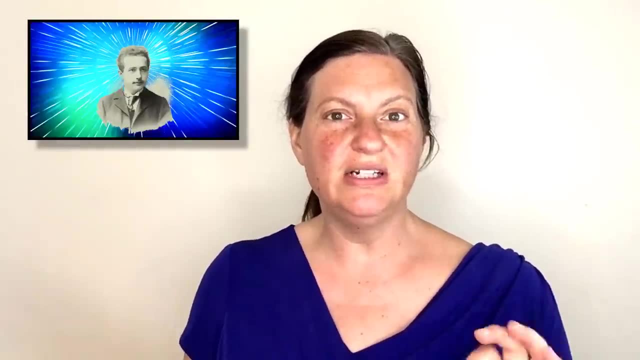 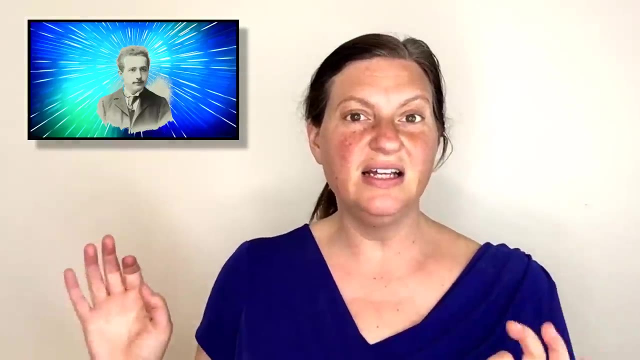 heard of her. In May of 1904, Mileva did not get another Leserelle as she had a boy, Hans Albert. Despite what you might have read or heard, Einstein enjoyed his job as a patent clerk, finding it, quote unquote- uncommonly diversified and pretty easy, In fact. Einstein later recalled: 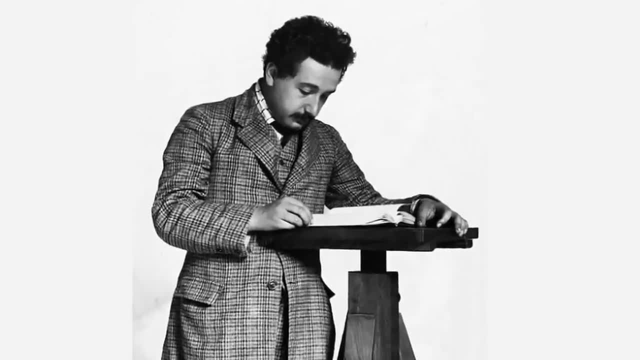 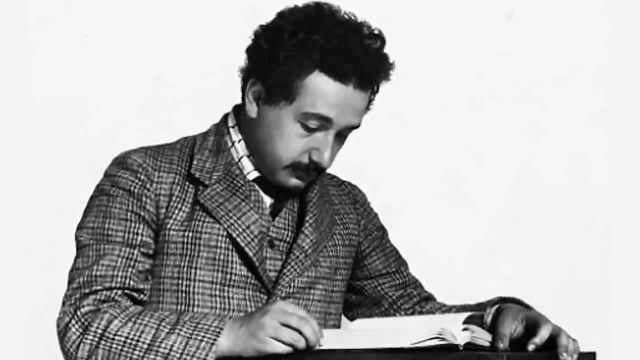 that he was able to quote, do a full day's work in only one or two hours, and the remaining part of the day I would work on my own idea, but when anyone came by, I would cram my notes into my desk drawer and pretend to work on my office work. In this way, the Einsteins kept up with the latest research. 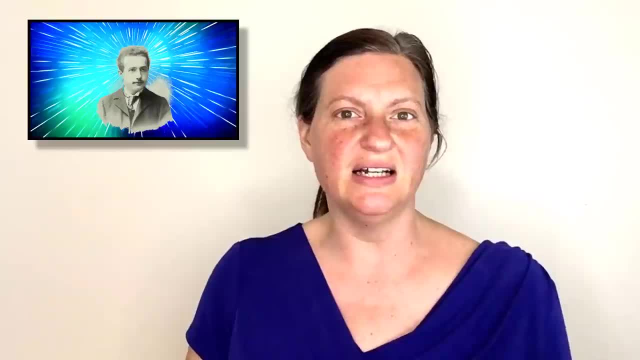 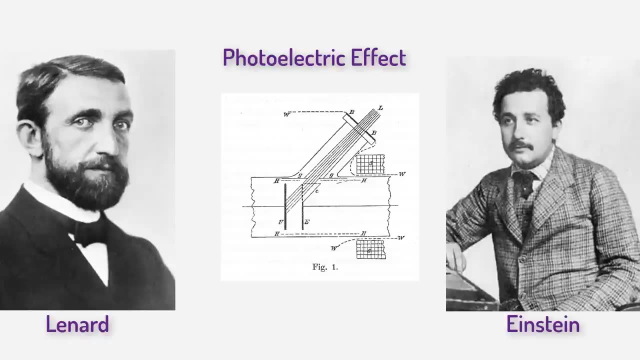 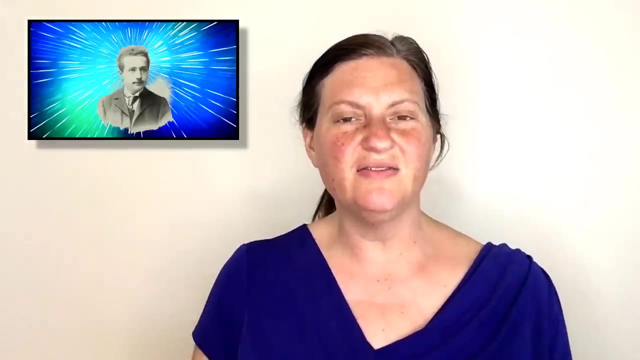 and Albert at least had a lot of time to think of new ideas. At around this time, Einstein read that Philip Leonard had conducted a new experiment on how ultraviolet light creates electrons in the photoelectric effect that Einstein called pioneering See. Leonard had the very clever idea of adding an 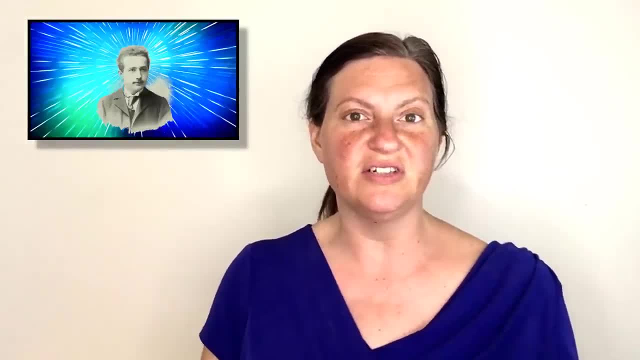 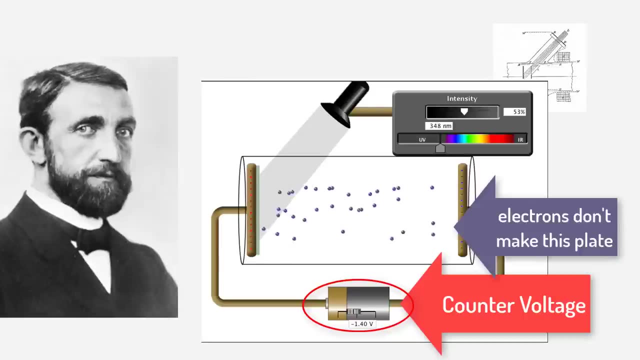 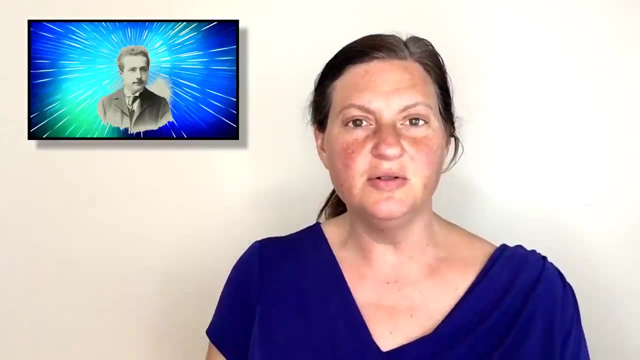 extra voltage the wrong way, which he called a counter voltage, so that the electrons freed by the ultraviolet light would be pushed back towards the irradiated plate, as Leonard said, quote: in the same way as a stone thrown upward falls back to the ground. Leonard knew that the voltage to stop 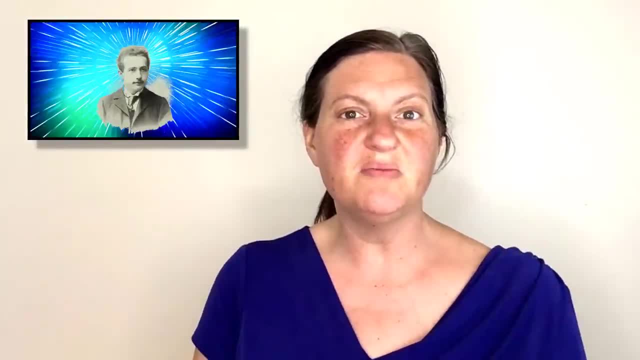 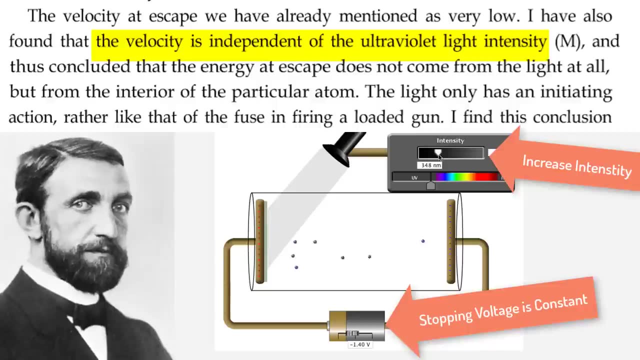 the electrons from reaching the other plate could tell him about the top energy of the freed electrons. then Leonard found something truly startling. the top speed of the freed electrons was unaffected by the intensity of the light. Leonard decided that the energy of electrons did not come from the light. 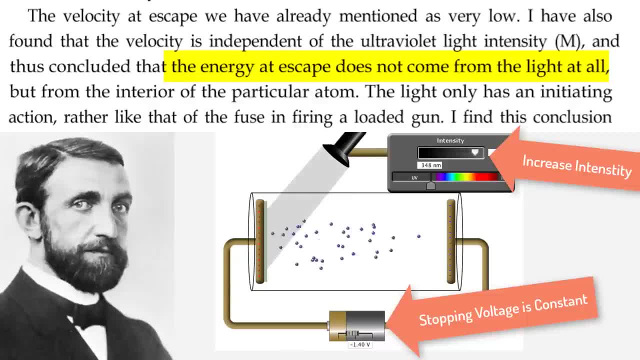 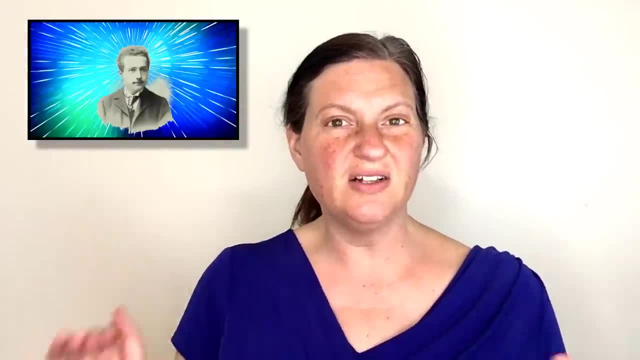 but instead the light acted like a trigger to relieve electrons form, the world's negative energy, the inherent energy of the atoms, like quote the fuse and firing a loaded gun. this triggering theory seemed like a good solution and even as late as 1909 it was written as one of the 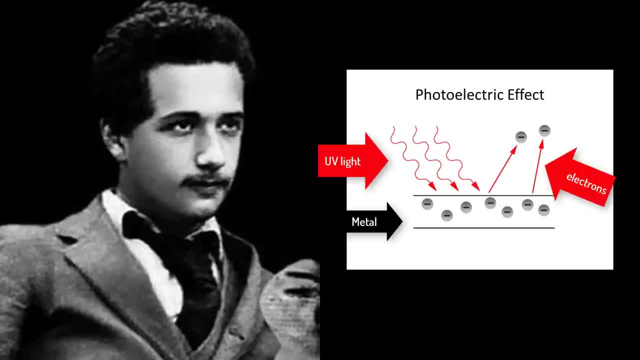 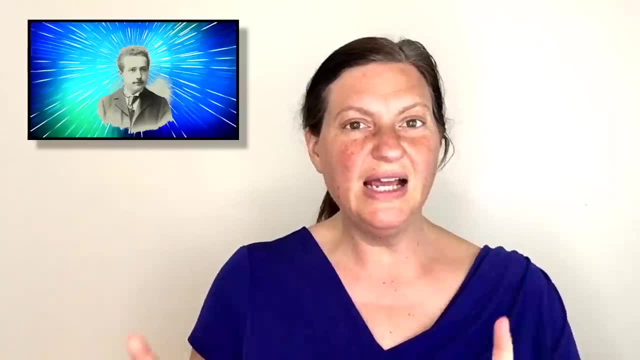 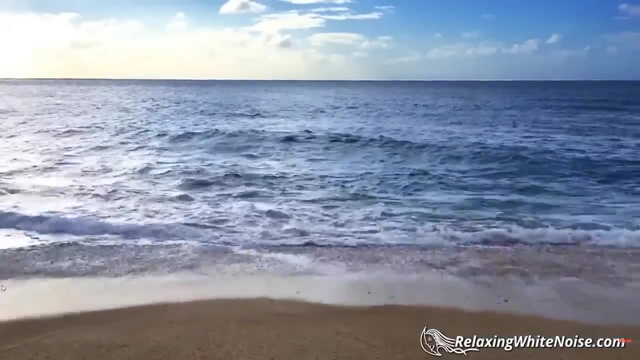 generally accepted truths of physics. however, in 1904 or so, einstein had a quirky thought: what if the energy of the electrons did come from the light, but the light didn't act like a typical wave? see for a typical wave, like a sound wave or water wave: the higher the intensity, the greater. 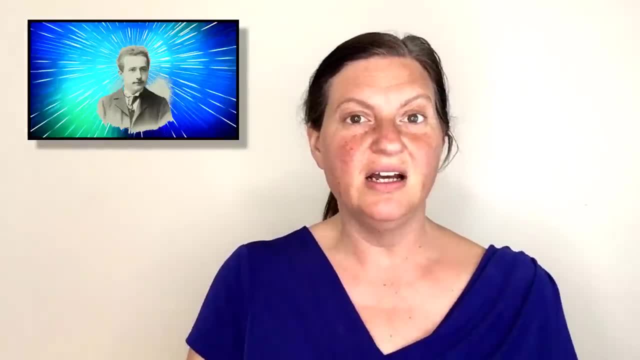 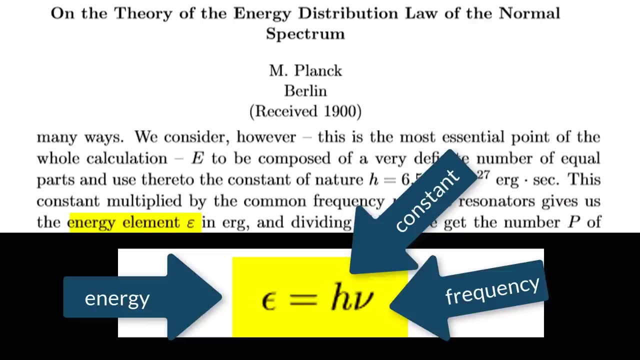 the energy, so more intensity. ultraviolet light should lead to higher energy-freed electrons, but that's not what leonard had observed. however, einstein remembered plank's paper, where plank assumed that light was created in little energy packets, with an energy that depended on the 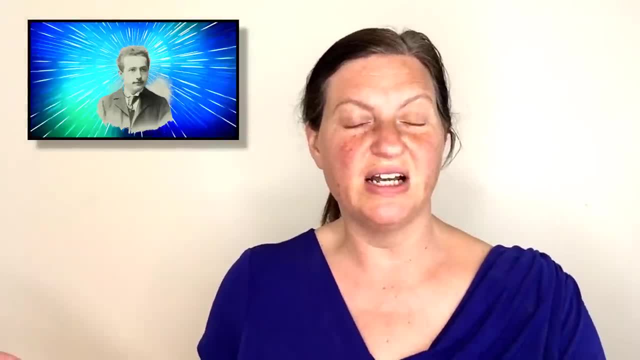 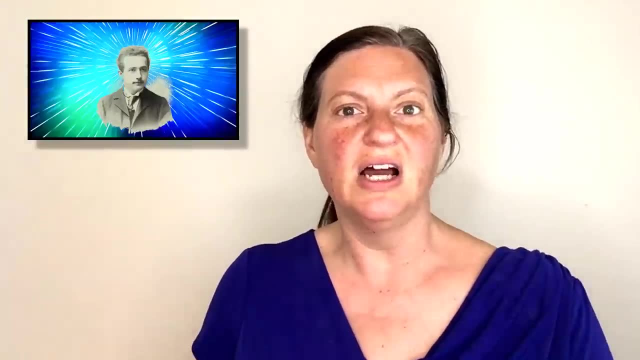 frequency of light. now, plank just did this as a math trick, but einstein started thinking: what if it was light that was created in the frequency of light that depended on the frequency of light, literally true. what if light was composed of tiny little particles that could only be created moved? 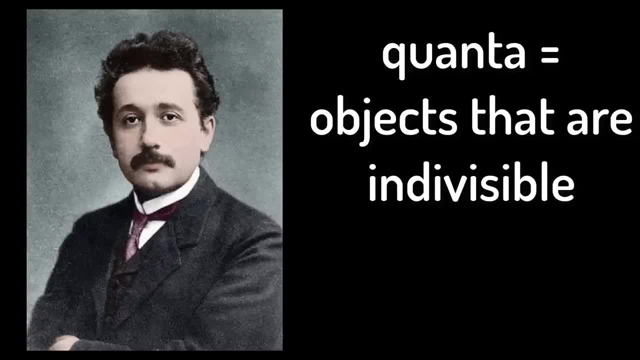 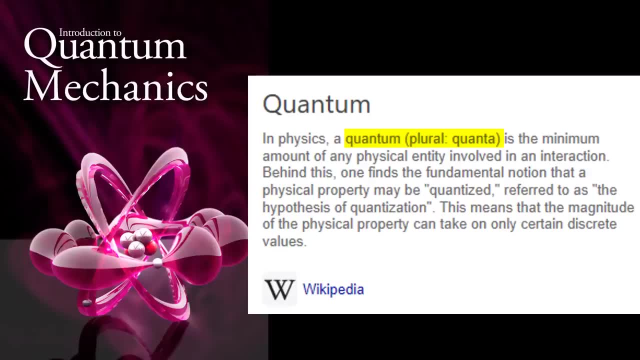 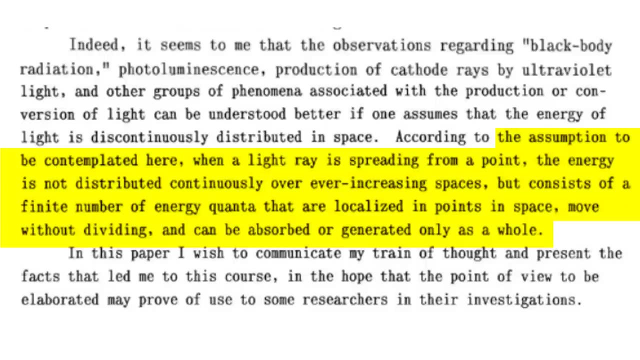 or absorbed as a whole. einstein called these particles quanta, which is a word for units that are indivisible, which is why this branch of physics is called quantum mechanics, quantum being the singular of quanta. in 1905, einstein wrote- quote- the assumption to be: 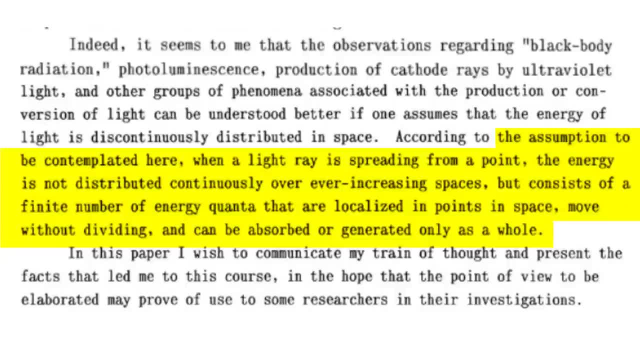 contemplated here is that when a light ray is spreading from a point, the energy is not distributed continuously over ever-increasing spaces, but consists of finite number of energy quanta that are localized in points in space, move without dividing and can be absorbed or generated only as a whole. this has been called- quote- the most revolutionary sentence written by a physicist. 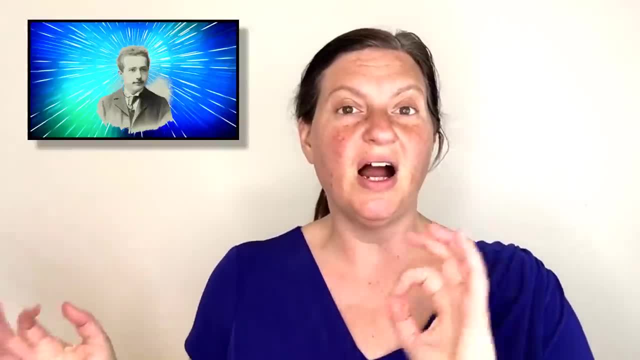 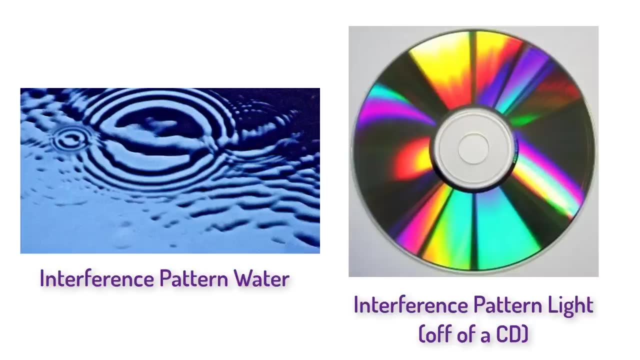 of the 20th century. before this, paper items were either waves or particles. this was the first proposal that they could be both. light has free energy and light has no free energy. and light has frequency and creates interference patterns like a wave, but is composed of little energy packets. 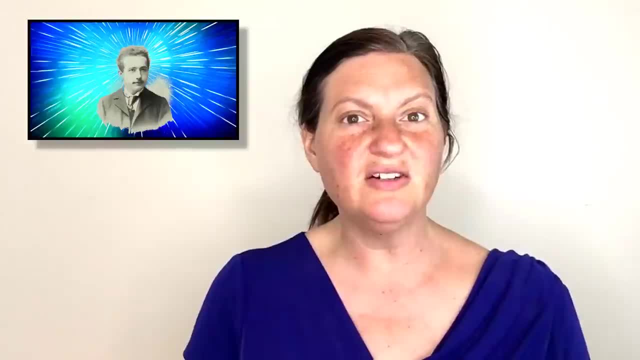 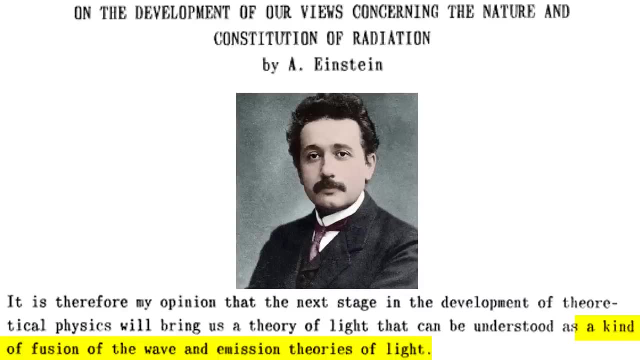 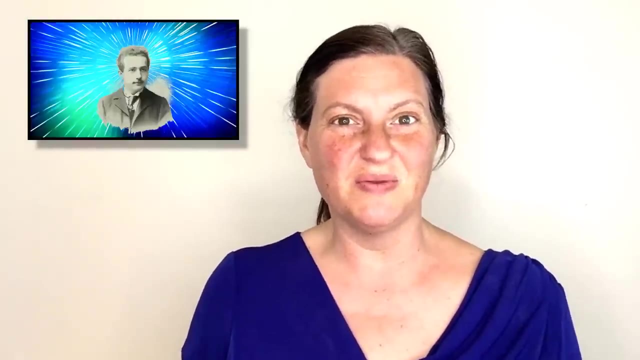 that cannot be split in two, just like you can't split an electron in two like a particle. later einstein described it, quote- as a kind of fusion of the wave and particle theories of light. if this makes your brain hurt, you are not alone. even einstein was never really comfortable with it. 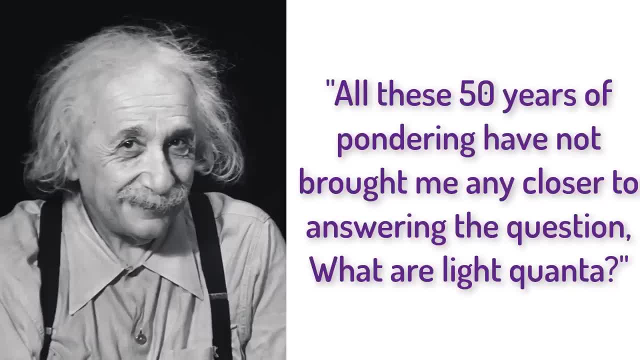 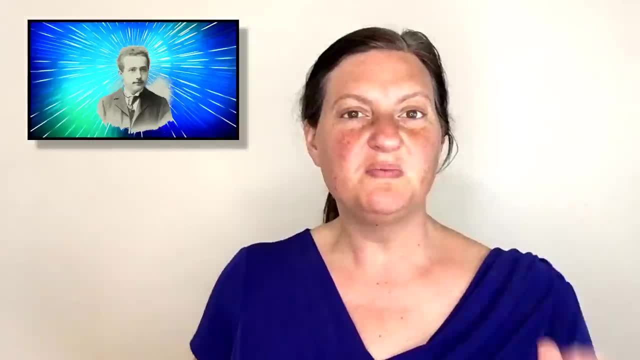 and in 1951 he wrote his friend beso quote: all these 50 years of wandering have not brought me any closer to answering the question: what are light quanta? despite not really getting what light quanta are, einstein found that this counterintuitive idea 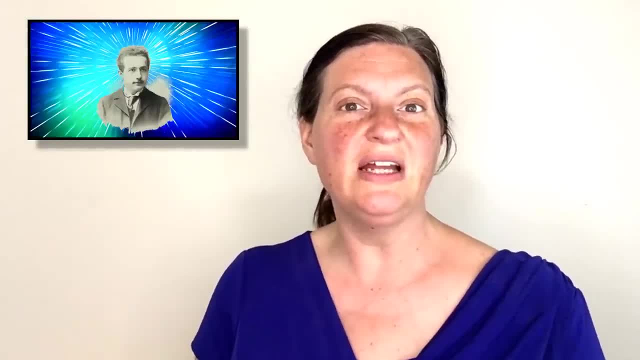 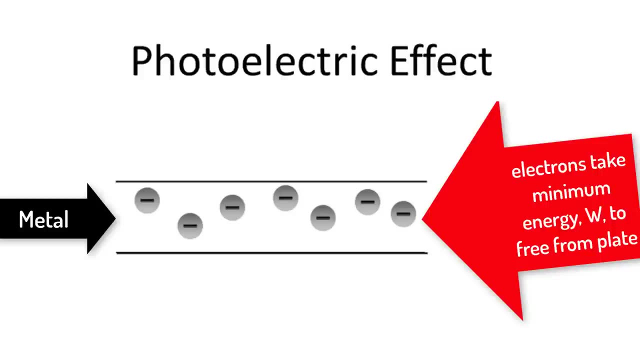 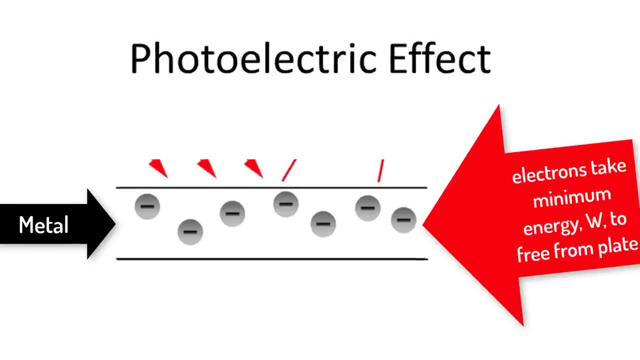 of treating waves like a bunch of particles could explain all sorts of phenomena, including the photoelectric effect. einstein decided that in the photoelectric effect, electrons on the plate are stuck to the metal by electric forces and can only be removed by giving them a certain amount of. 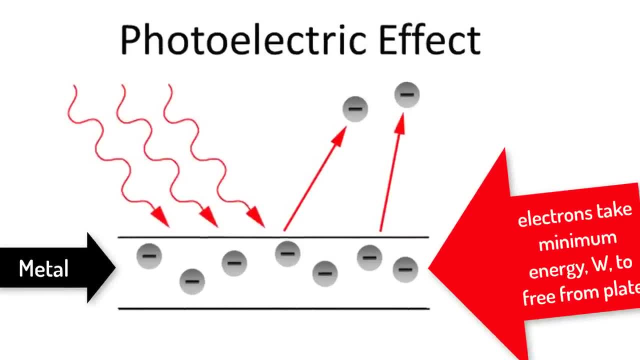 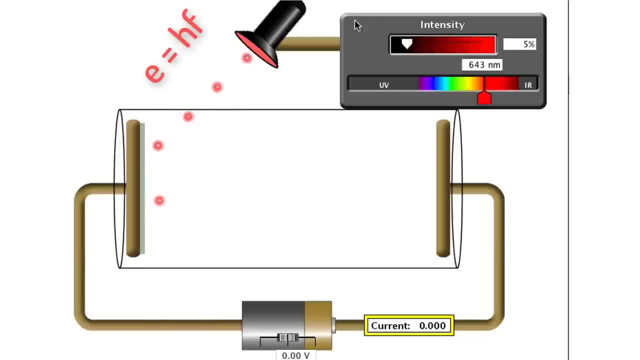 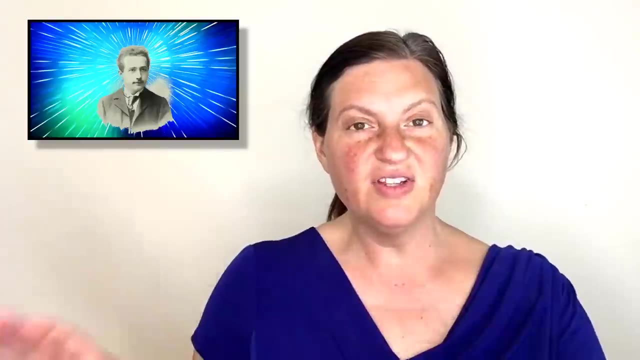 energy, absorbing the energy of the incoming light. einstein then postulated that the light came in little energy packets, where the brighter the light, the more packets. but the individual light packets, now called photons, all have the same energy. if the frequency is too low, the photons of light 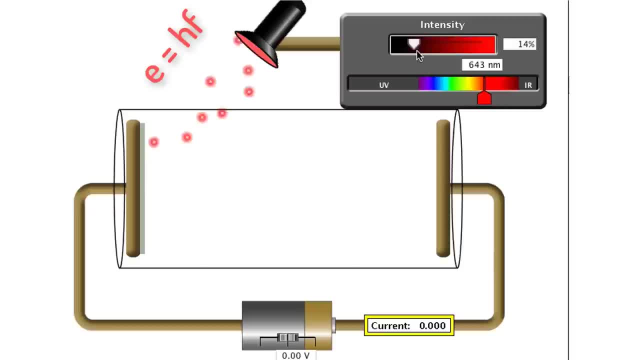 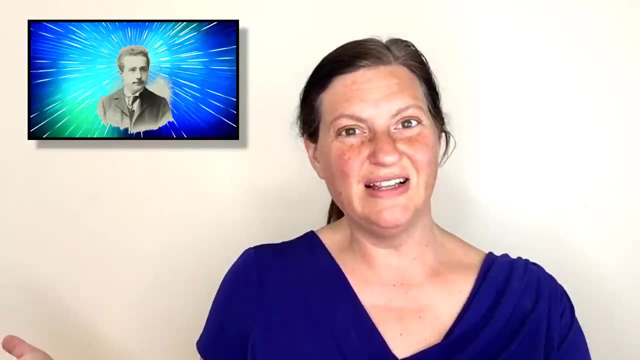 have less energy than the binding energy of the surface electrons to the metal and no electrons will be freed from the plate, no matter how many packets you throw at the plate. this is why you need relatively high frequency light to create the photoelectric effect. also why uv light creates sunburn and visible light does not above this threshold the more intense. 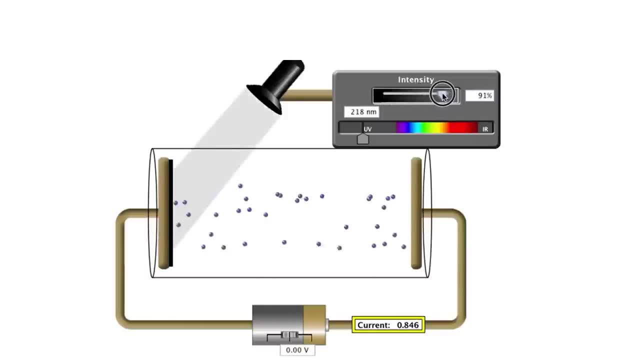 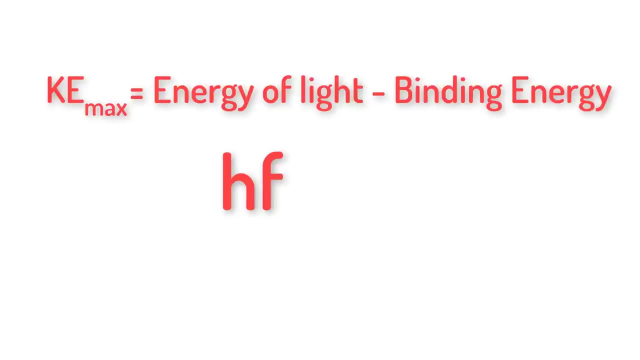 the light, the more electrons are freed. the electrons all have the same maximum energy, the energy of the photon of light minus the minimum energy to free the electron. according to planck's equation, the energy of light is planck's constant h times the frequency. and according to einstein, the minimum energy to free the metal is a constant of the. 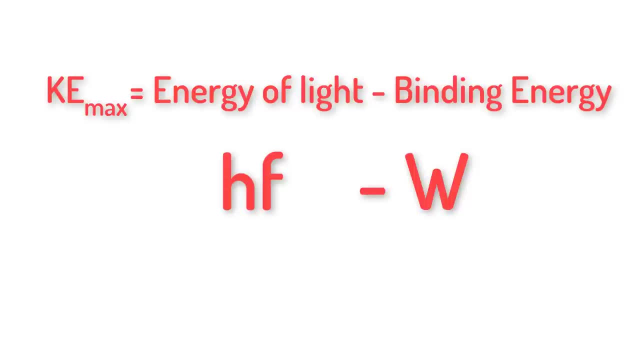 metal. einstein also knew from energy conservation that the voltage to stop all the electrons from moving to the other plate times the charge on the electron equals the maximum kinetic energy of the electrons. thus einstein created the equation for the photoelectric effect. interestingly, in this equation for any metal there are only two variables in the 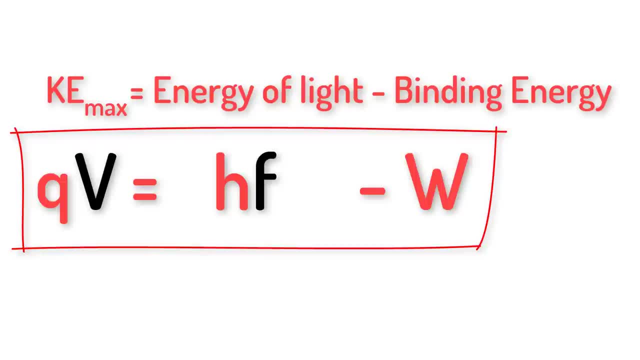 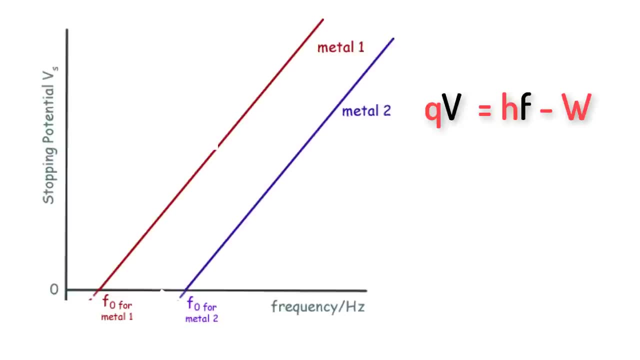 equation the stopping voltage and the frequency. therefore, einstein theorized that if you graph the stopping voltage versus the frequency of light, you should get a straight line, no matter what material you use for the plate. even more impressively, the slope of that line can give you planck's constant h. einstein found an experimental way to prove that light comes. 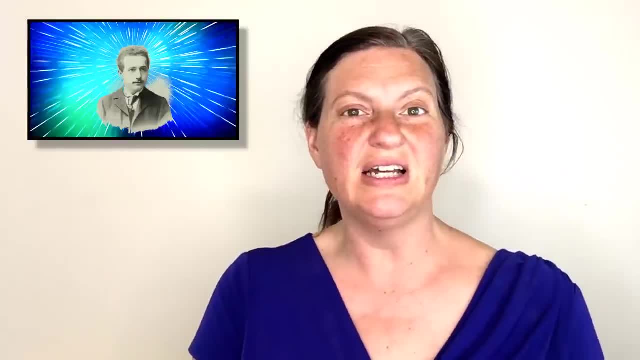 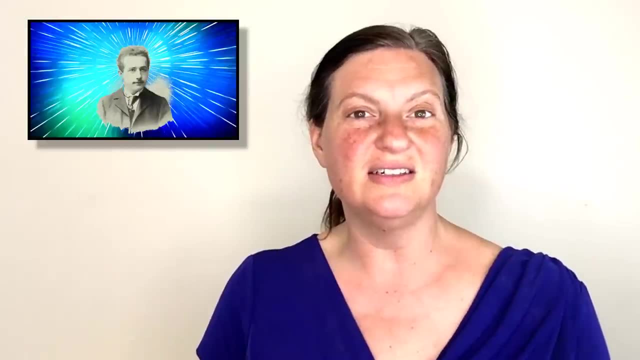 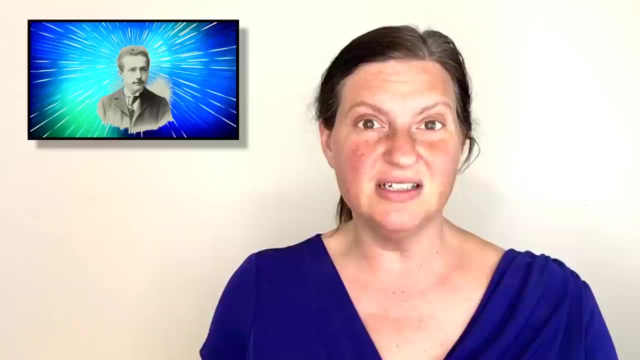 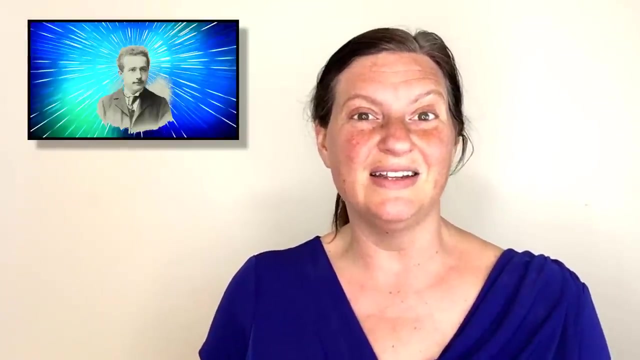 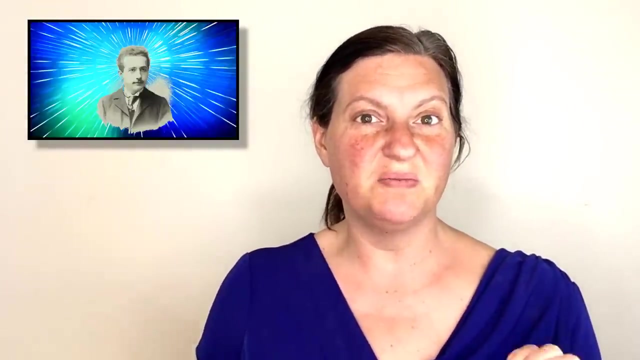 in little energy packets with an equation equal to constant times, the frequency of light and the voltage of light. the e even found a new way to find a universal constant of nature. you think an experimentalist would have jumped on this. however, the experiment was ridiculously difficult to do and no one was much interested in what an annoying patent clerk, third class, had to say on the issue anyway. in fact, it took nine years for any experimentalist to successfully do this experiment, at which point the scientist who did it, robert millikan, of oil drop 5.. 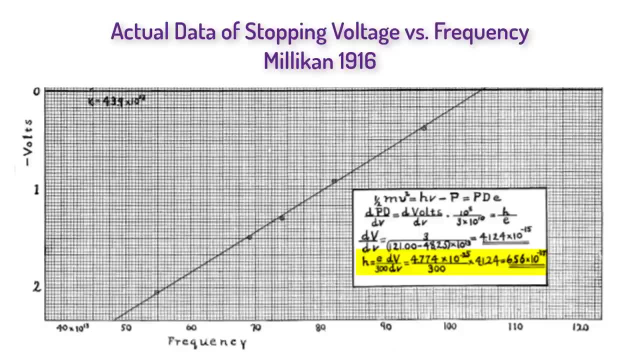 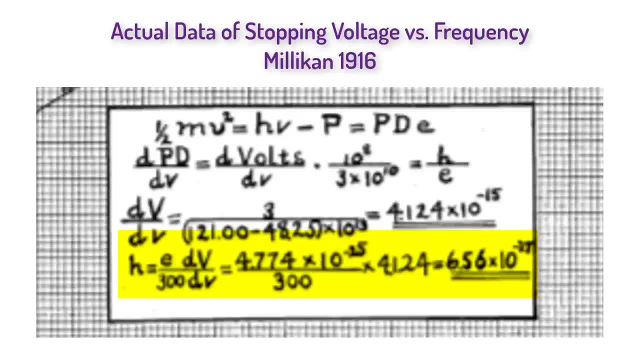 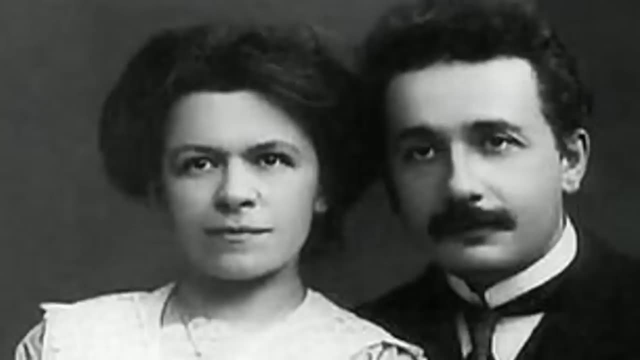 fame found. his results were, quote: a complete success of the Einstein equation, Although Millikan continued to reject what he called the bold, not to say reckless, theory behind it. A comment about Mileva: in all this, is clear that she helped her husband with his papers, at this time, as sometimes. 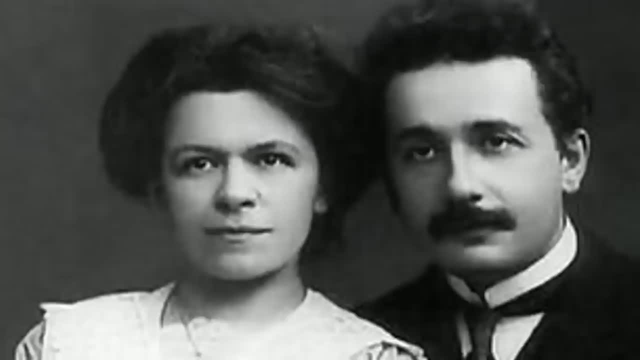 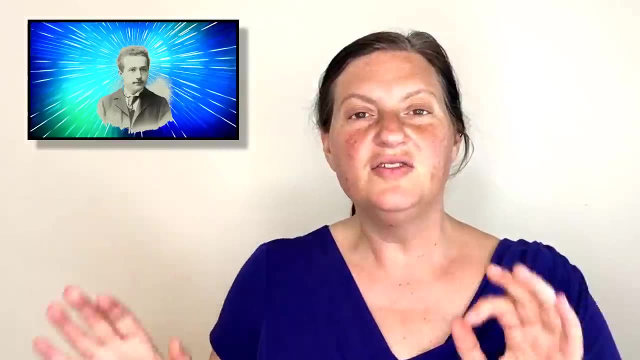 both Albert and Mileva called it our work in letters to each other, And Albert had also told Mileva's friends quote: I need my wife. She solves all the mathematical problems for me. There are no mentions, however, of Albert attributing any ideas to his wife. Is this because she made no? 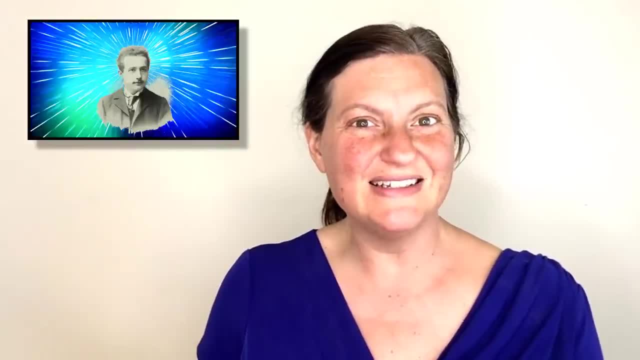 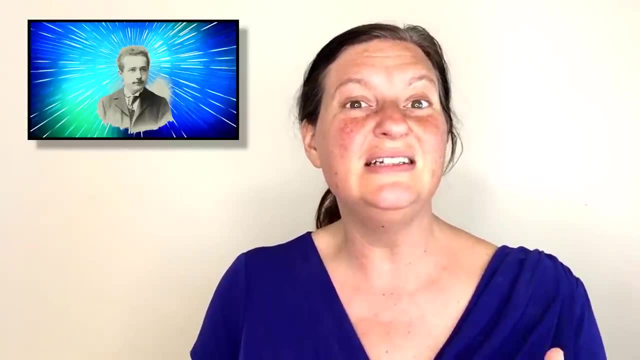 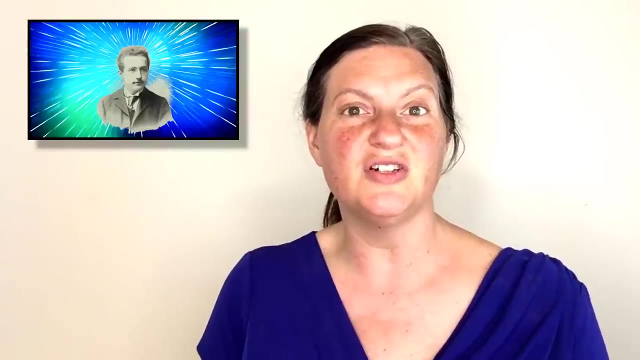 contributions, Or was it because he was kind of sexist and he considered her basically his student, as he affectionately called her, and didn't feel like her contributions needed to be mentioned? This was how it was portrayed in the mostly excellent 2017 television show Genius. 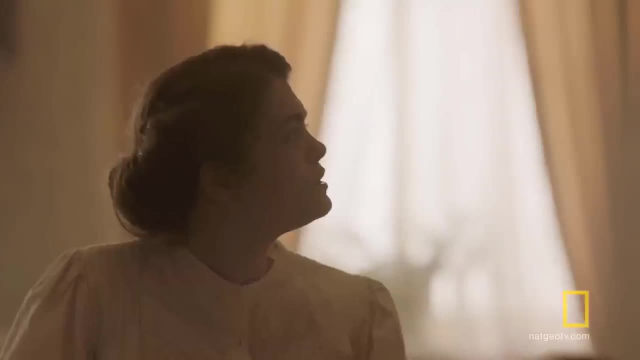 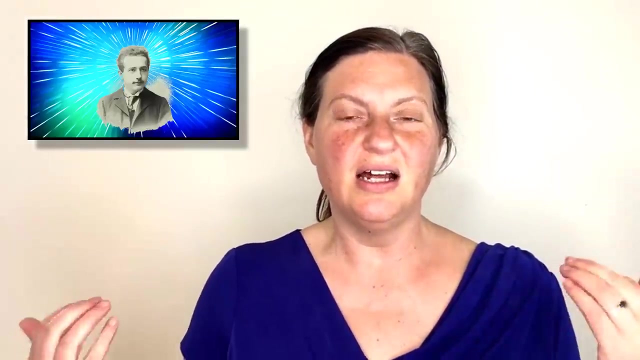 You thanked Michela. Of course I thanked him, But I've helped you with so many papers but you never thought To put my name in any of them. It never occurred to me. It also should not be discounted that Einstein was trying to be recognized in 1900s Germany. 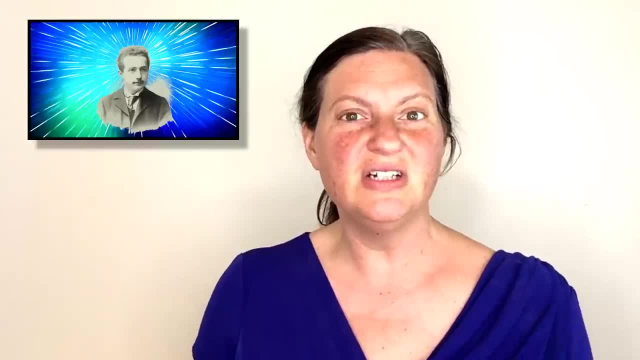 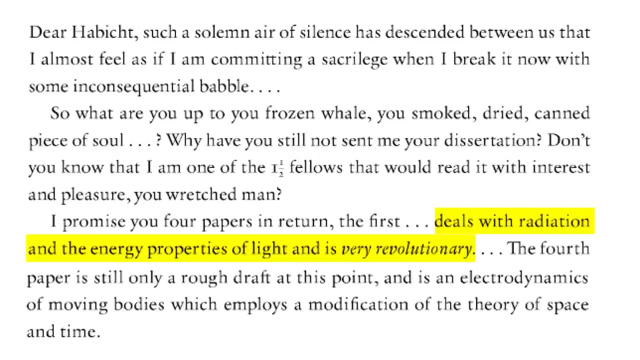 not a place where one would be respected for mentioning the contribution of one's wife. Anyway, as I said in the beginning, Einstein thought correctly that this paper was very revolutionary and therefore was not surprised to find it didn't get very far at first. 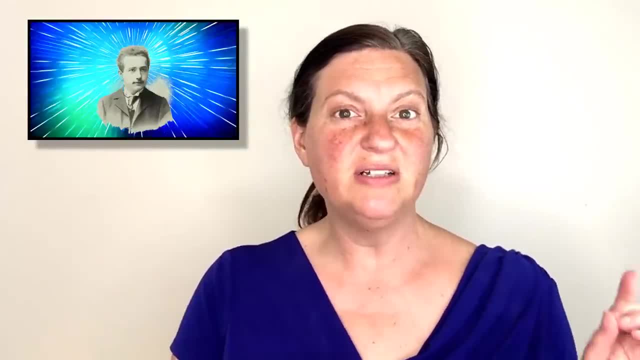 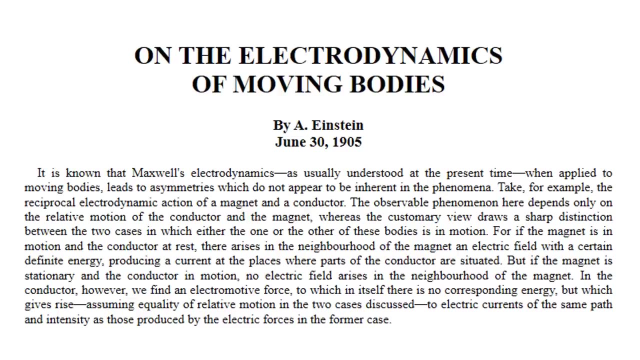 He had higher hopes for his next paper on Brownian motion to prove the existence of atoms, And that did get published, but it didn't go very far. His next paper was on a strange idea called relativity. That was the paper that slowly 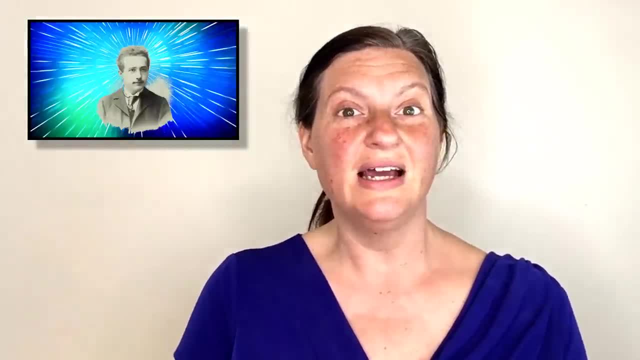 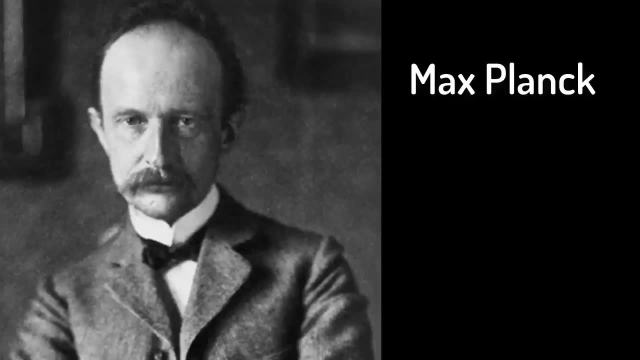 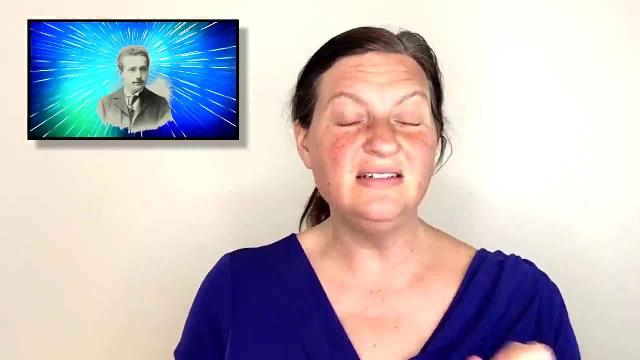 got the attention of some prominent scientists like Lorenz and even Planck. Strangely enough, Planck loved relativity instantly and fought against quantum mechanics that Planck himself accidentally initiated. In addition, that same year, Einstein published an addendum to his 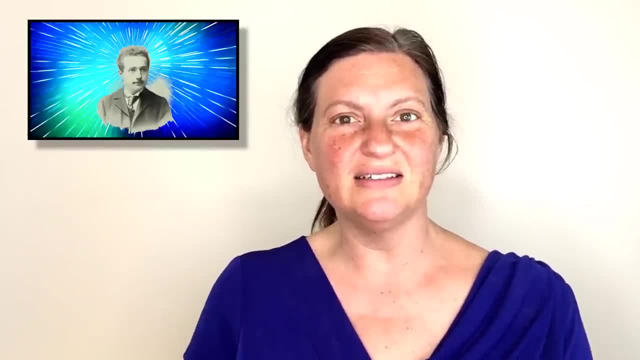 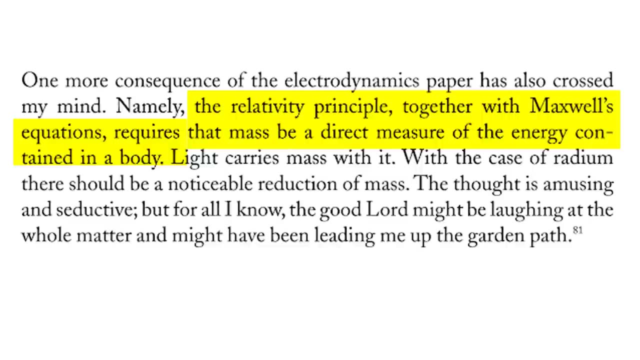 relativity paper. He wrote that Einstein was not interested in relativity. He was interested in the idea of relativity, The idea that the relativity principle, together with Maxwell's equations, requires that mass be a direct measure of the energy contained in a body. In other words, 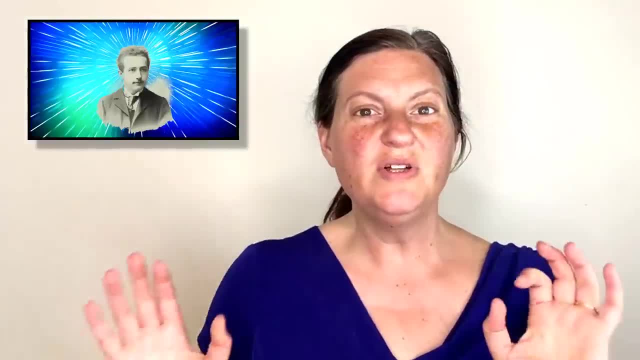 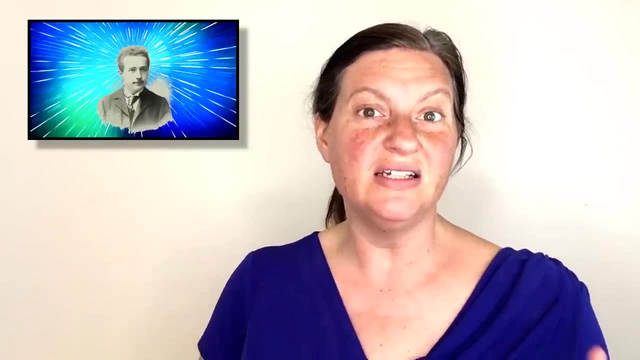 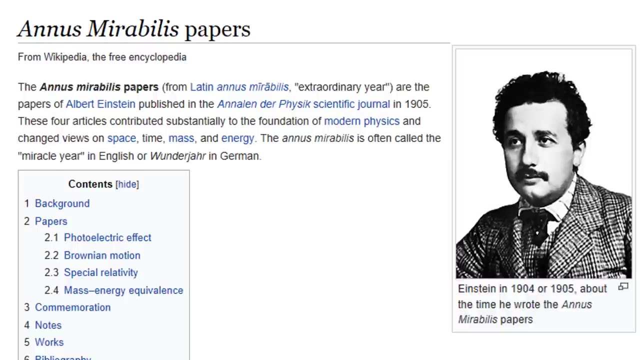 Einstein published that E equals mc squared. One would think that any of these papers would have catapulted Einstein into scientific starving. After all, that year 1905 is considered so influential for him. This is called a miracle year in science, Like 1666,. 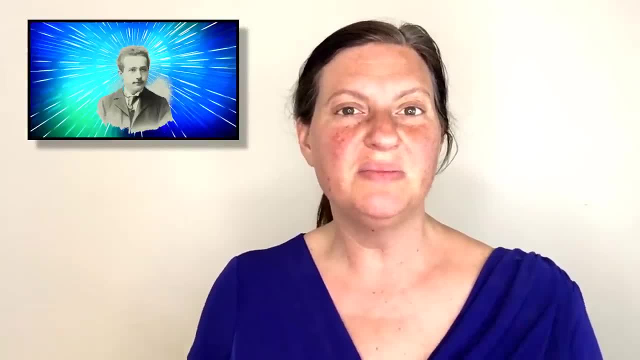 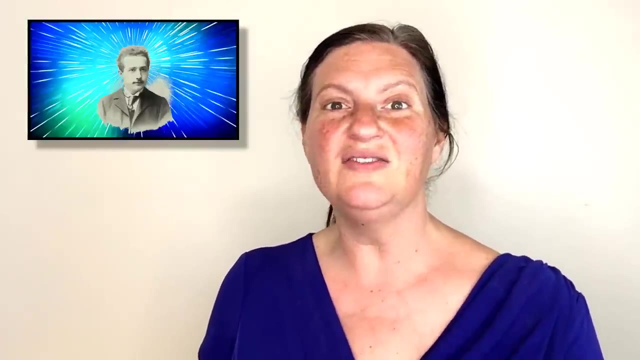 newton. however, it was a really slow burn. it took him until 1909, four years later, for him to even get an associate professor position. and it wasn't until the next year, 1910, that he became famous among scientists, not for relativity, but for quantum mechanics. in fact, einstein's 1911 talk.